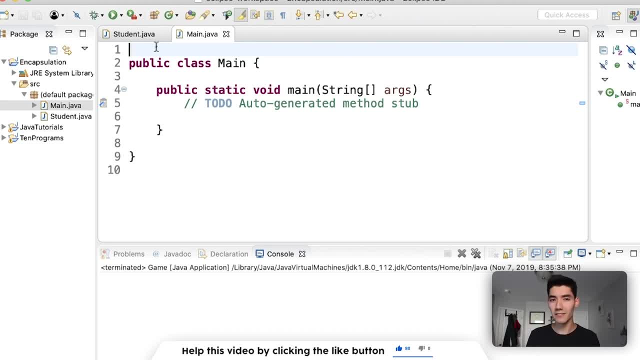 a pill. everything is inside the pill, But for encapsulation in Java all the setting of variables of a class is inside a method. So we'll just go into our student class and this represents a student object or just a student in general. All objects in Java have attributes and things it can do. So let's describe the student. 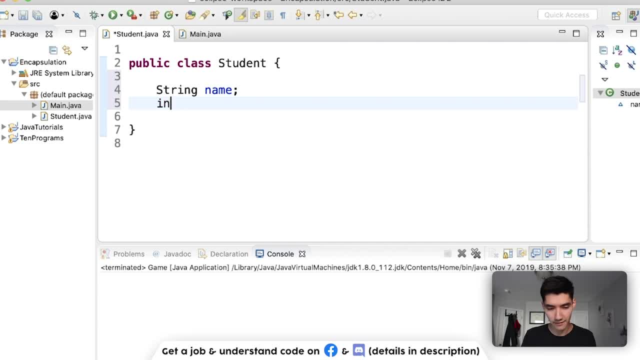 here, Say it has a name, and let's say they have an age, And we could go on to add methods that say what the student can or cannot do, like enroll in a class method or whatever. But the methods we want to write are for encapsulation, which is setting and retrieving the variables. So name is 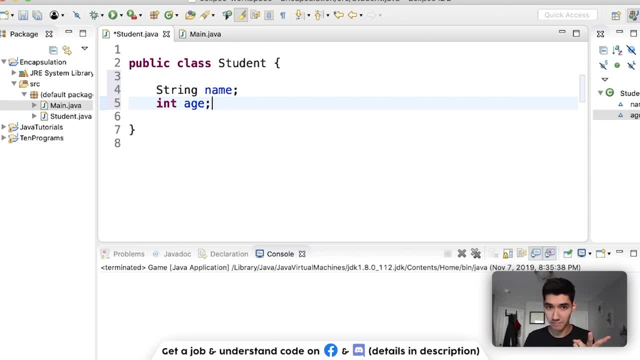 going to have two methods called get name and set name, And age is going to also have the two same methods, but set age and get age. Now, we'll get to that in a second, but I want to show you why this is important. So if we tried to use our student here, we'd have to make a student, So like. 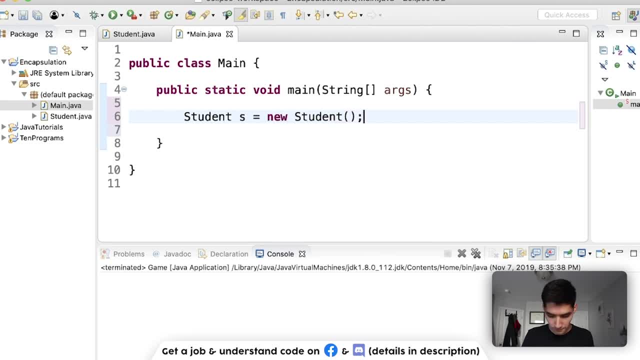 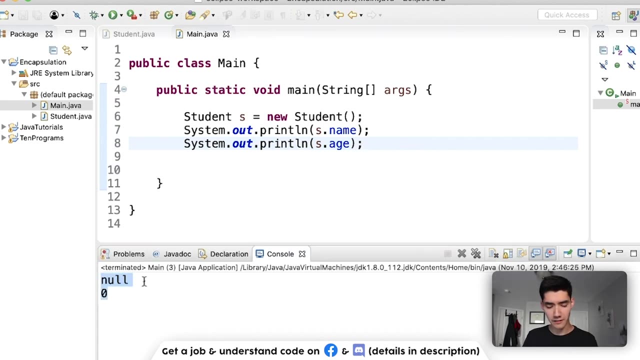 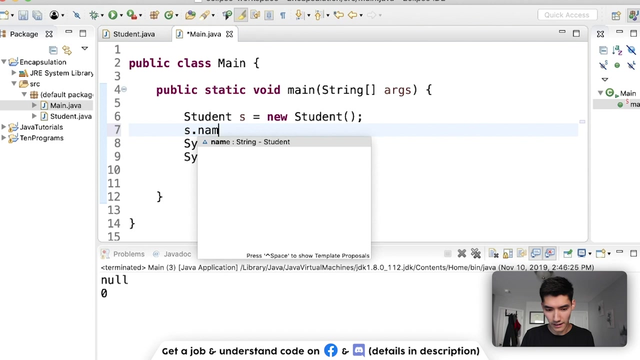 student s equals new student And we can print out those variables: s dot name And s dot age. Right now it's null and zero because they're not set to anything. If we wanted to set the name and age this way, we would have to do s dot name equals, say, Tommy, and s dot age equals 17.. 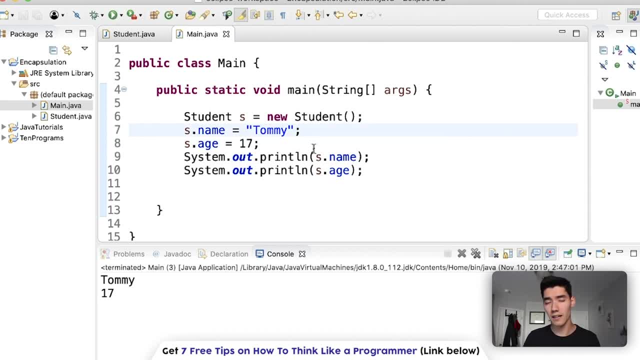 Save and run, But this isn't a good practice in object oriented programming, because what we really want to do is we just want to call methods that do this for us, instead of having to type out: equals this, equals this all the time. so the way we use encapsulation is to get around this. 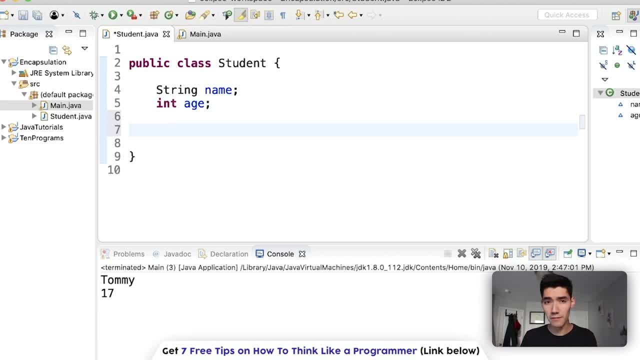 and we use getters and setters, so let's make those now. every method has a few keywords in front. these methods are going to be public, for whoever wants to create a student can access these. so we're going to say public. we're not going to include the static keyword, because static means. 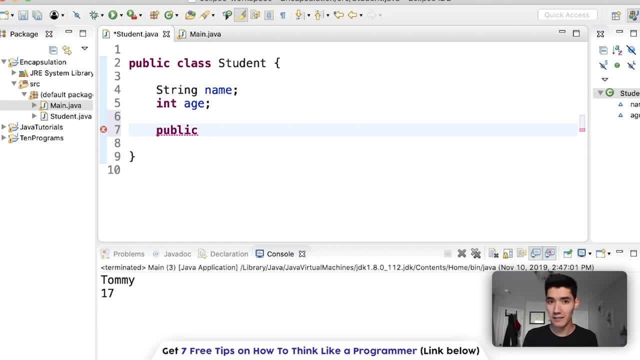 you don't have to make an object to call a method. but in this case we are going to make a student object to call this method. so we're going to skip the static keyword, we're going to set the name and in this case it's not going to return anything because we're just setting it. so 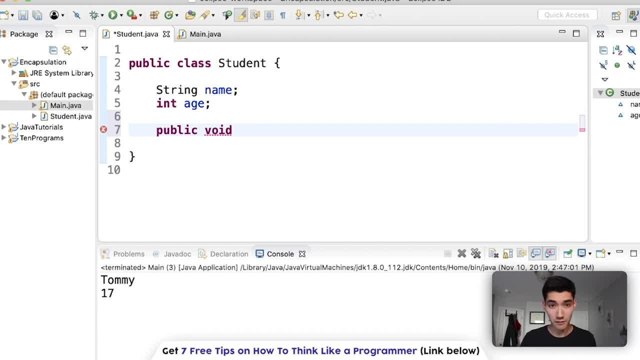 if we don't want to return anything in the method, we just type void. the name of our method will be set name and we'll pass in our new name in here and all this method is going to do is say name equals new name and that's it. so let's try to test this out. we'll call set name. 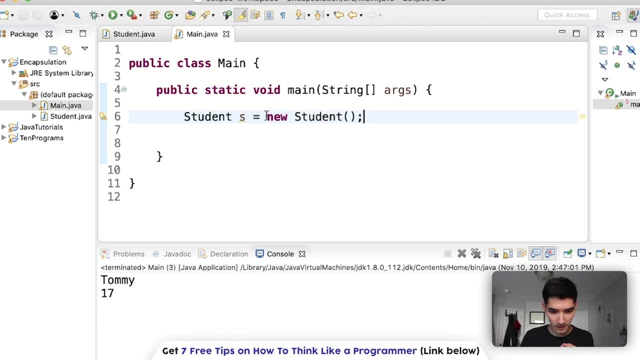 from the main method and try to set this name. so we have our student. we're going to do s dot to bring up everything the student knows and can do. in this case it knows the age and name, but since we added set name, it also knows set name and we'll add: let's do a different name. 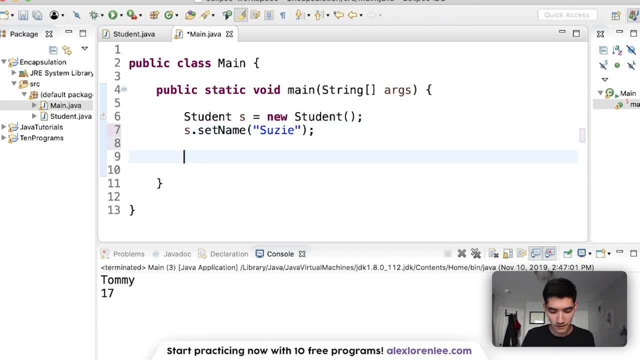 about susie, and then we'll print out what the actual name is, save and run and we get susie. so basically, what we're doing is we're creating a student object, s, and s knows everything inside of here. so when we put an s, dot, set name susie. 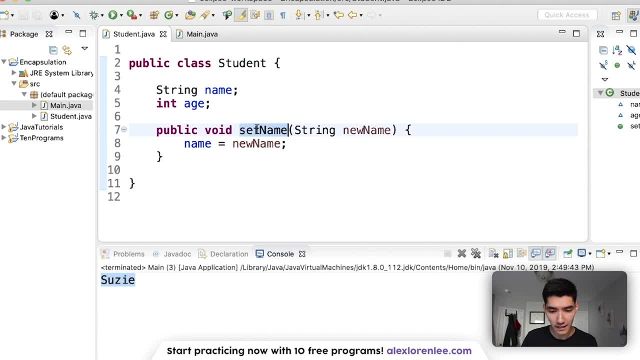 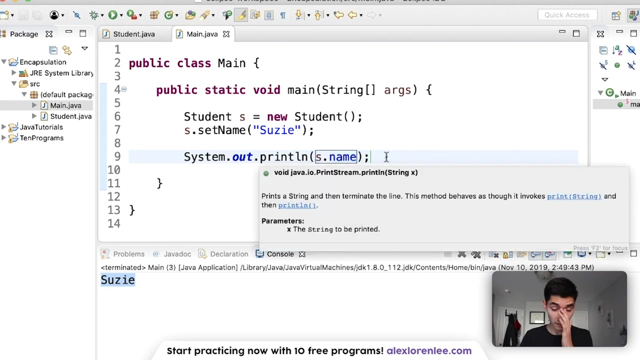 in the parameter. it knows that there's a method called set name with a string parameter and it goes in here: sets name equal to the new name which we passed in as susie and then so when we print out s dot name, since it's set, we print out susie. now this might be kind of like. well, we could set it with the equal sign. 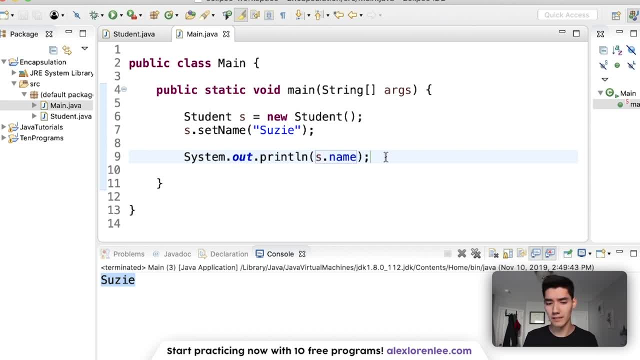 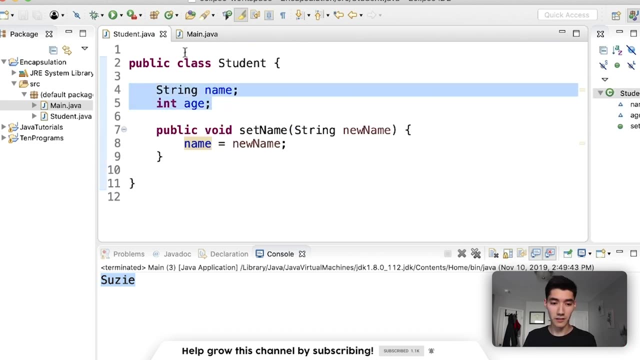 or we could set it with the method what. what's the big deal? why do we really need to do this? well, the point of encapsulation is to abstract the variables from the user to make it simpler to use the object. so, in reality, these would not be shown to the user. 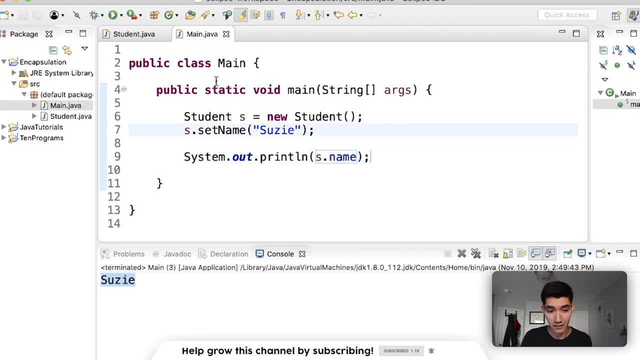 we would not be able to do s-dot-name or s dot h, so these should actually be private. they should not be shown to the user, so these need the private keyword. now, if we tried to run this, we get an error, because now when we do s dot the age and name. 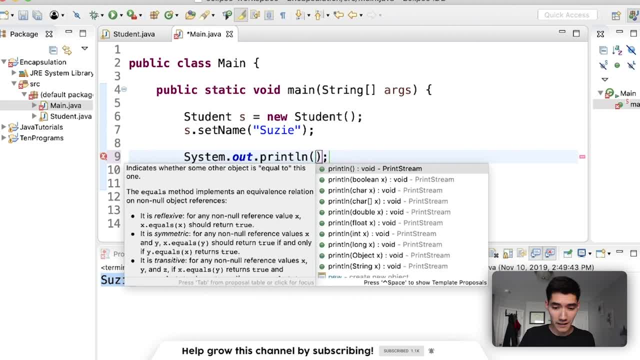 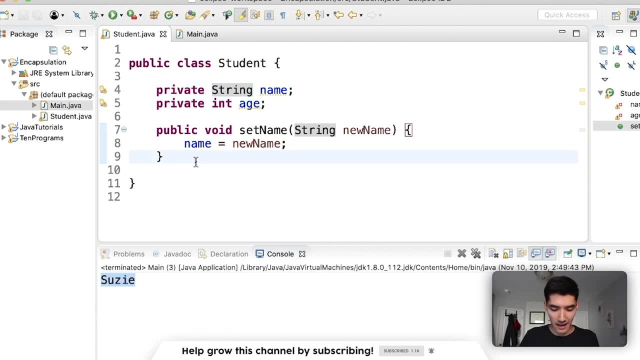 don't show up because they're hidden. they're private. so now what we have to do is we have to create a get name method, since we no longer have access to these, and again, the whole point of all this is to make it simpler for the user, so they don't have to deal with the variables as well. 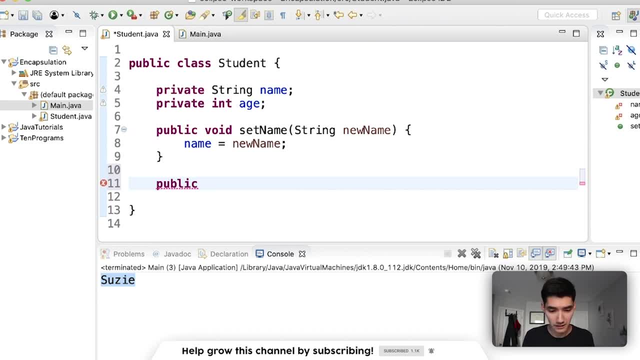 so this is public because the user is going to use this um. it is going to return the name. because we're getting the name, we're going to bring the name back to whoever is using it. so name is a string, so our return type is string: get name. since we're just retrieving the variable, this method is not going to be useful if we have 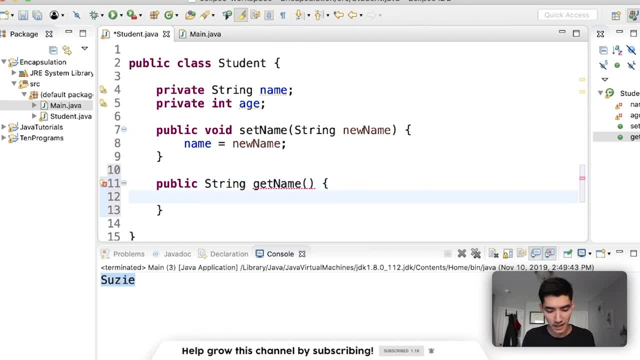 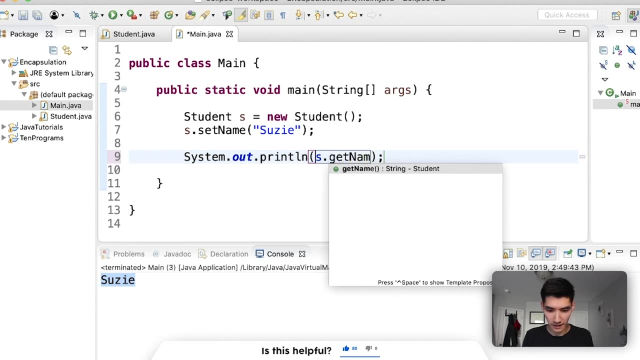 to pass something into it. so we're not going to pass anything in and we're just going to use a return statement to return that name into the method call. so if we did get name here- oh, excuse me, s dot get name. since it's public, we can see this method. we run this. 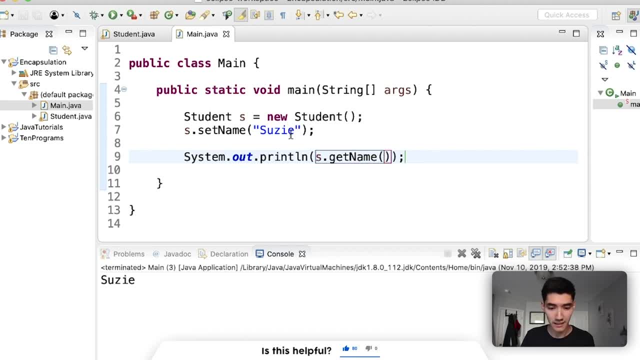 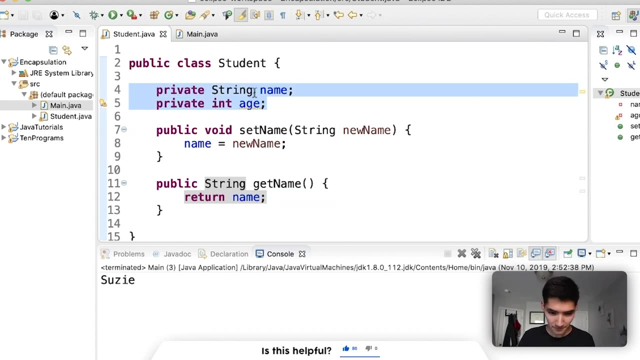 it does the same thing. we do s dot set name and then s dot get name, and this is basically encapsulation. okay, it's that simple: just making a set method and a set their latest service, a get method for the variables because they're private, to make it simpler for the user. so now, 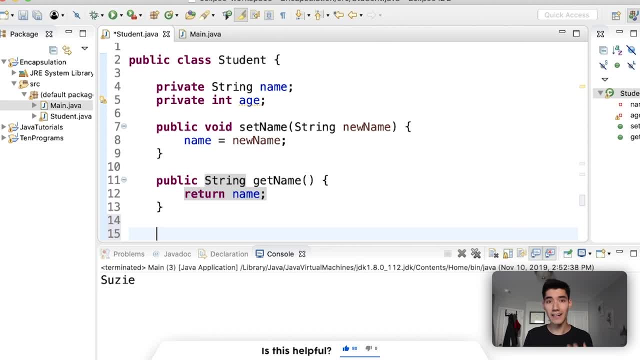 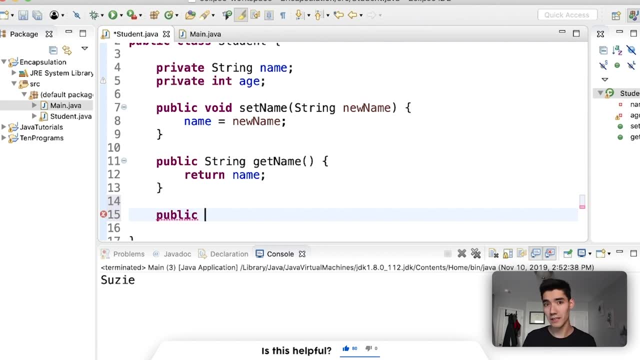 let's do this with age. let's make a set age method. this is going to be public to the user. since we're setting, we're not going to return anything because we don't really need to, so we'll just type void. we're going to set age and we'll just name it set age, because that makes 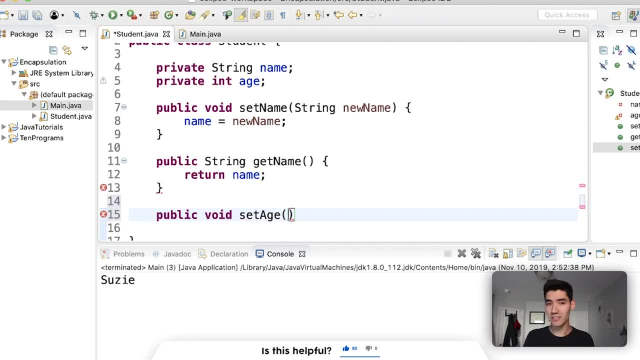 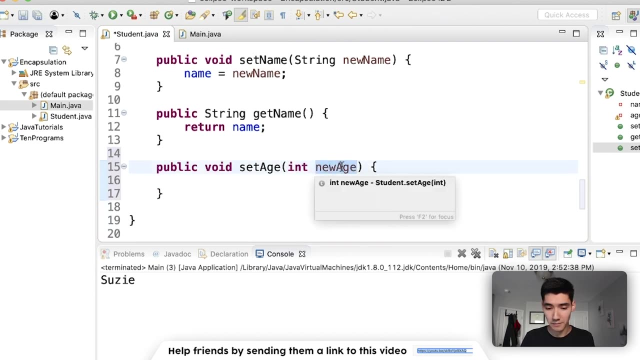 sense and we're going to set the name, set the age equal to whatever the user passes in. so to make it match up we've got to pass in an integer. we'll call it new age. if this um parameter name was the exact same as the variable name up here, you'd have to do: 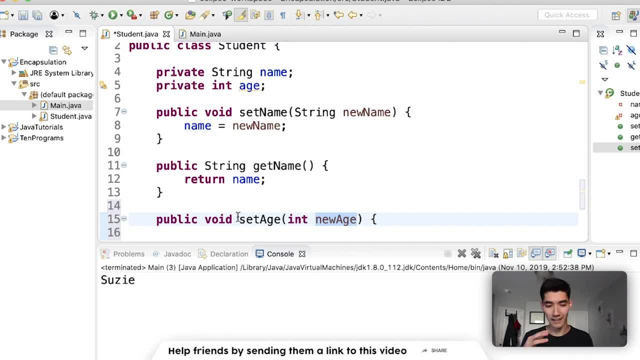 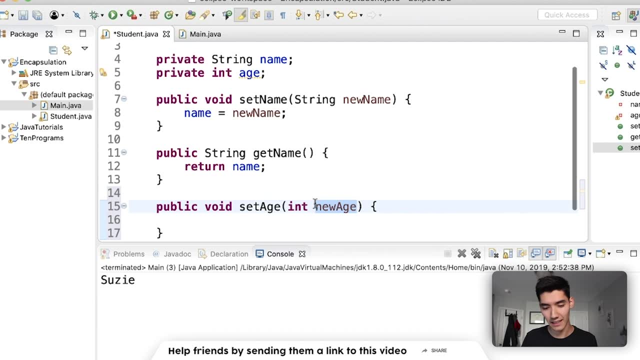 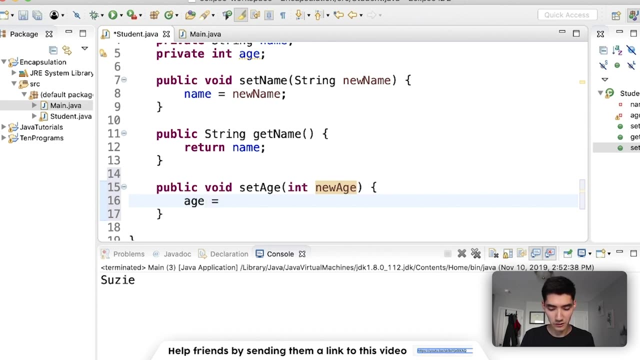 um, you have to use, uh, the this keyword to kind of get around it. you have to do this: dot name equals name or this: dot age equals age. i have a video on that if you want to check that out. but it's it's not necessary if the parameter names are different, so we'll just set age equals new age. 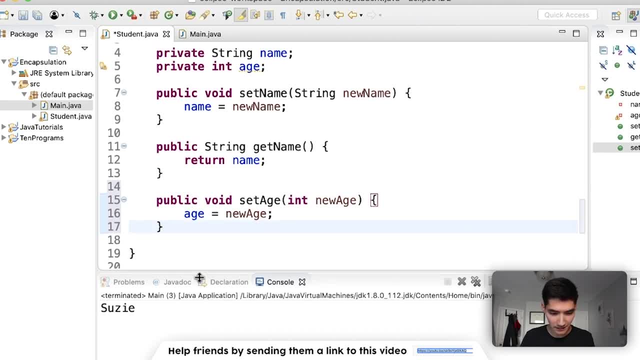 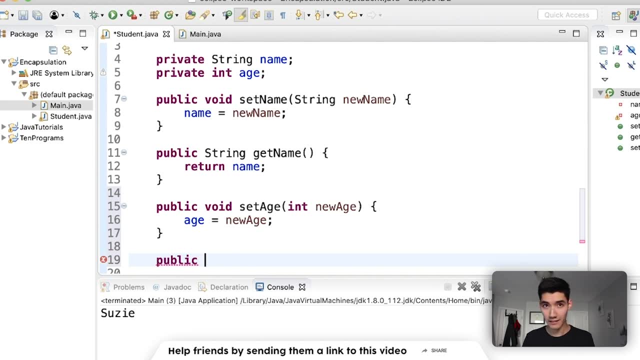 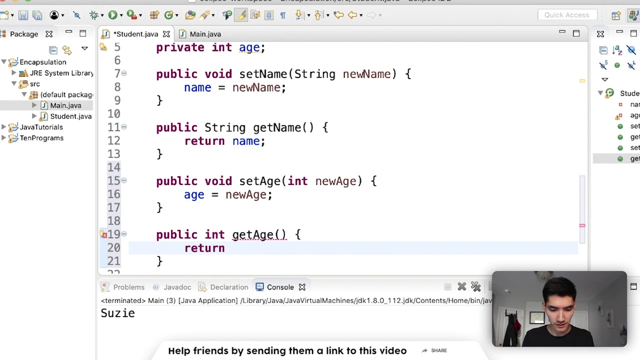 now we'll make the get age method- get age here- public because the user is going to use it. we're going to return an integer because we're running get age, so it has to be int called it get age, no parameters, because we don't need to, and then use a return statement to throw the age. 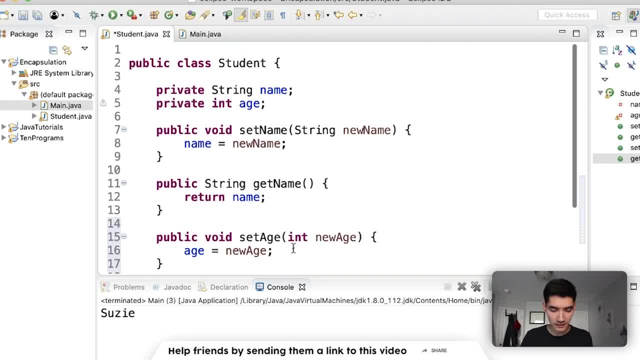 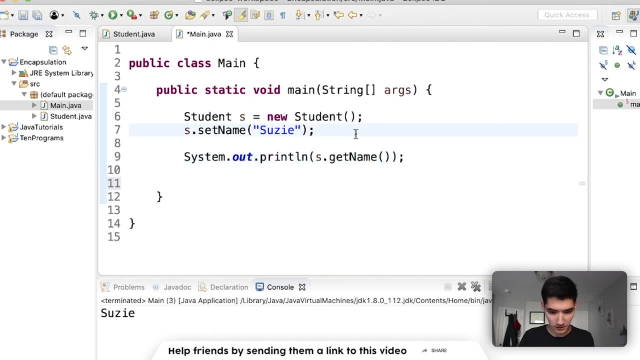 back at the user. so this is all the code, if you want to see it, and i'll go over this at the very end as well. um, we'll just do s dot. set age to what age this should be. should be 24.. and then we'll print out: 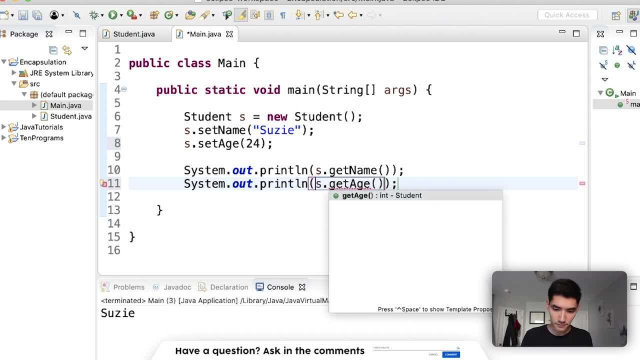 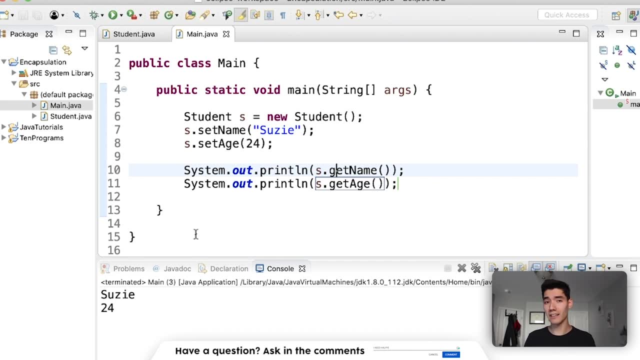 s dot get h. let me see, susie is 24.. so again, encapsulation is one of the simplest things in object-oriented programming. it's just that, since it's such a big word and teachers don't really know how to explain it to people who don't know what object-oriented programming is or are new, it just seems complicated. 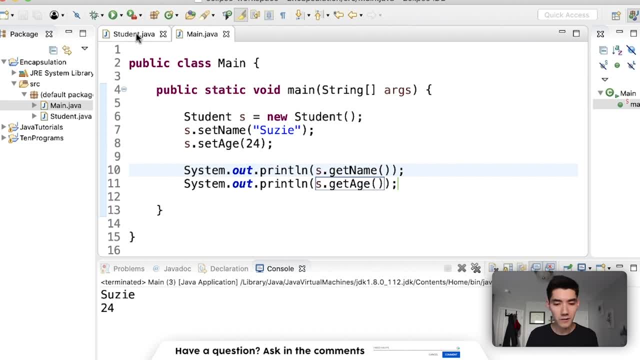 but in reality it's extremely complicated. so we're going to go ahead and do that and we're going to make a set name method and pass in a name. we'll say set name to the object and pass the name to the object. and pass the name to the object, um, and then we'll do a get name method which will 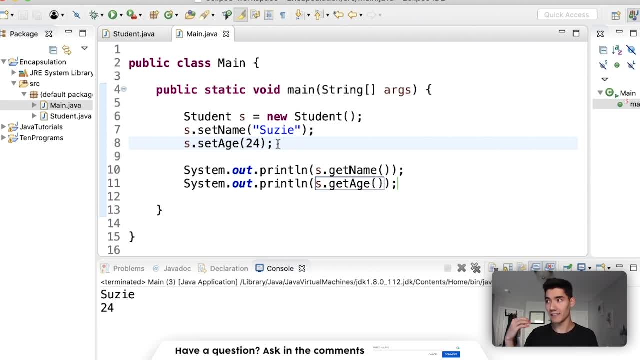 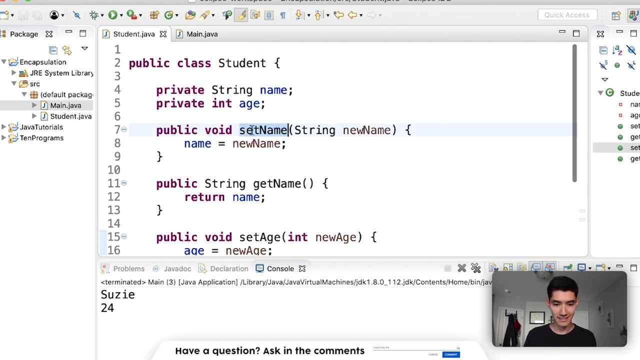 return the name. let's see, we're gonna take this method and we're gonna do it. this is a very simple method. it's extremely simple. all we're doing is making it simpler for the user of an object so, like the student object, we're allowing them not to have to deal with variables and to just set and get.